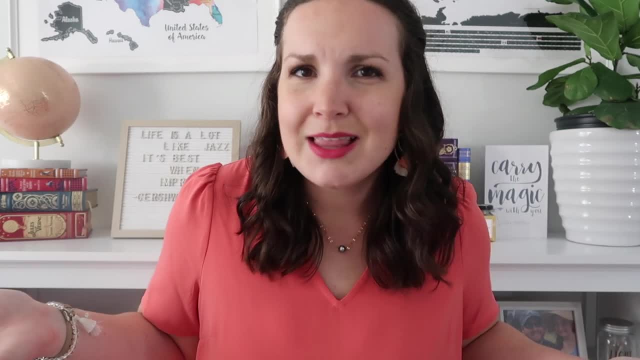 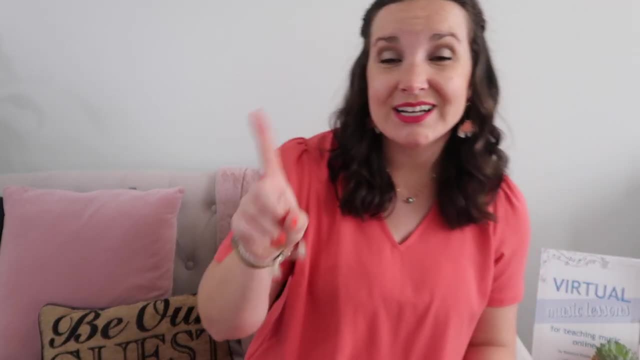 over there. Send me a DM or just comment on a picture and let me know what you love, because I'm always looking for new ones as well. Without further ado, let's get started. Let's hop right on in, All right. number one is going to be Hickory Dickory Dock. This is a really 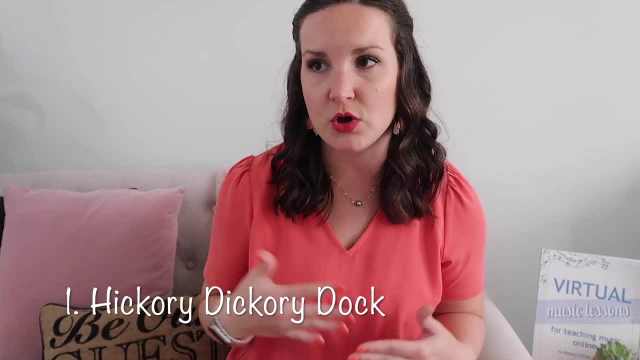 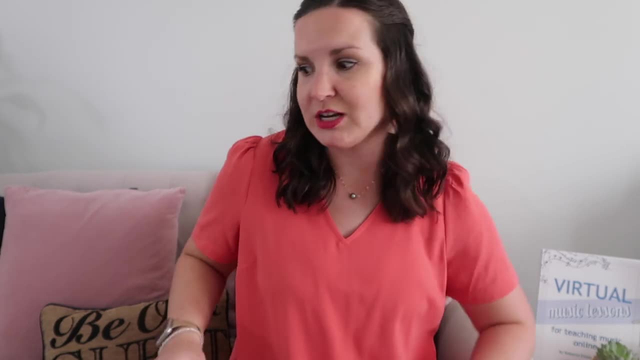 cute nursery rhyme that my kiddos love. I've also shared this with our second grade teachers and I made like a video to give them and they did this when they were teaching about time. But it's super cute and there are actions that go along with it. So for this one, we keep it pretty simple. We keep 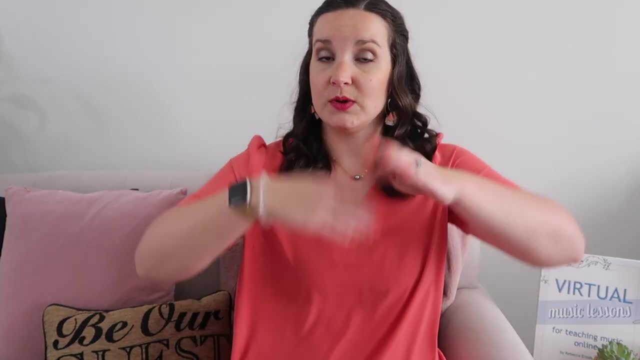 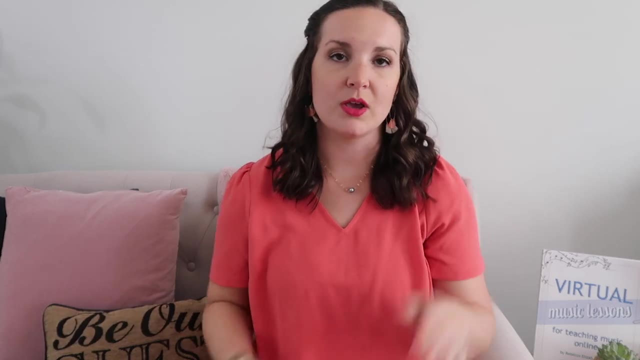 the steady beat and we go: hickory dickory dock, The mouse ran up the clock. The clock struck one, The mouse ran down. Hickory dickory dock, And then the clock strikes two, And then three, And we go all the way around and usually have the kids pick what time it's. 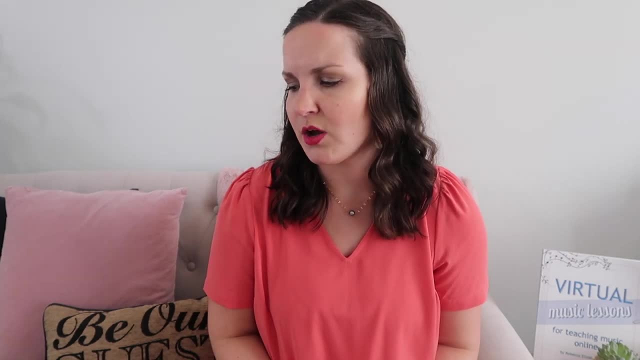 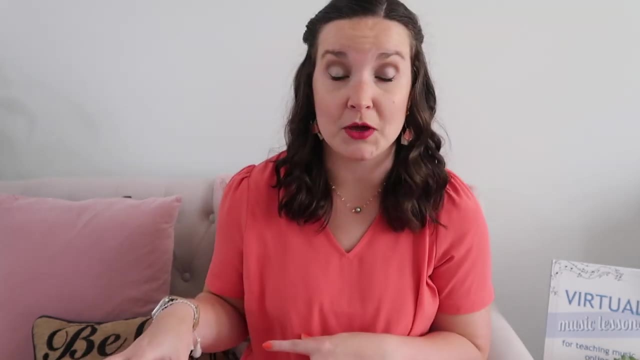 going to be to make it a little bit more fun, And it keeps them entertained for like a weird amount of time. So I actually have a free hickory dickory dock resource that I will leave a link below. I have a ton of freebies, by the way. I don't know why, but I have a lot of freebies that 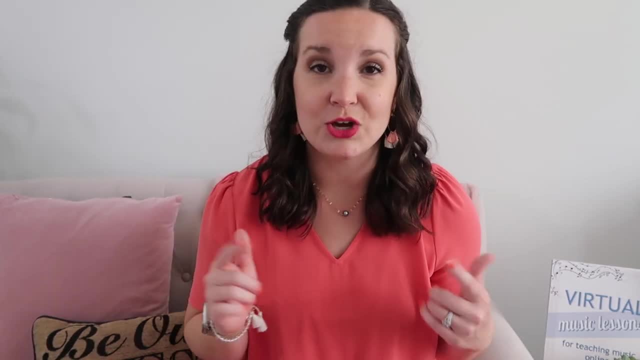 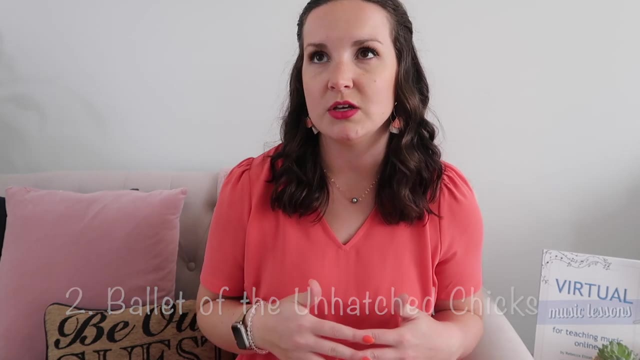 I'm mentioning in this vlog, in this video. So definitely go and check out the freebie down below. All right number two is Ballet of the Unhatched Chicks form. So I love teaching form. It's a really easy way to do movement. It's a really easy way to get kids listening to. 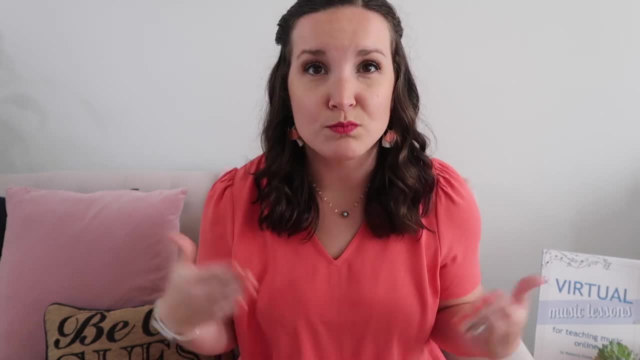 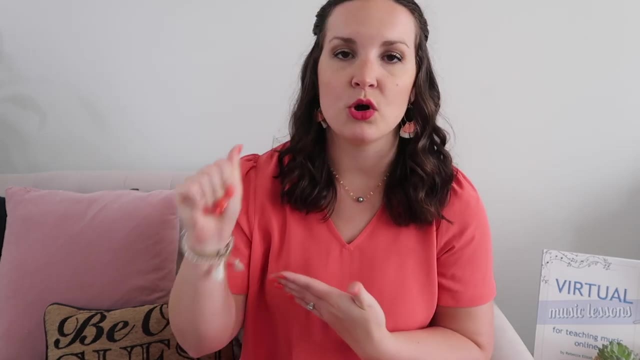 especially classical music, And Ballet of the Unhatched Chicks by Modest Musorski is one of my favorites. It's super cute. The form is A, A, B, A. That, by the way, is the sign language letters. I always do that first before we do anything else, And there are so many different things that you 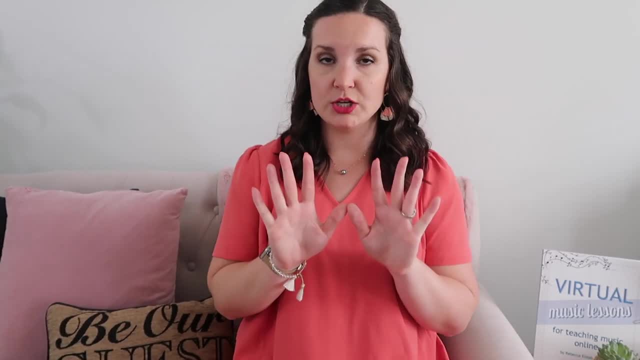 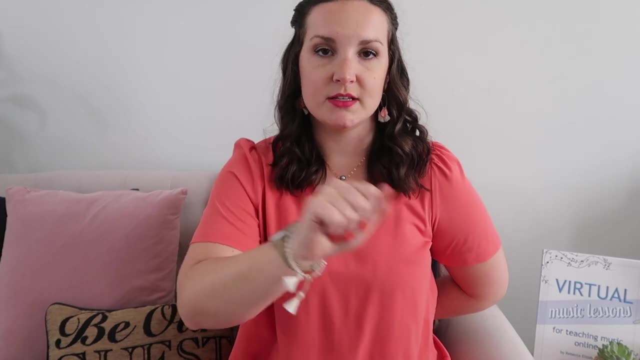 can do with this, But I like to use their hands. So what we do is you have A and B and you put them behind your back, And so when it's A, A comes out and it's the first little chicken He goes around. 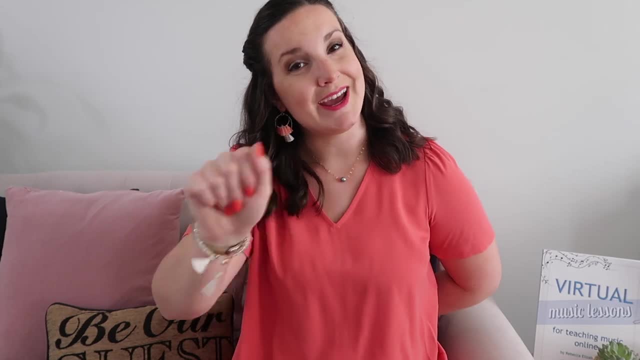 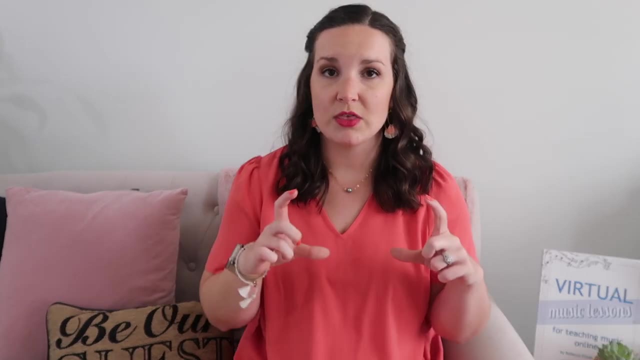 he goes back. he comes back out because A dances all around, goes back, and then B comes out and moves. B goes back and A comes out. You can also do this with like little cutouts. I've done that with like chickens in different colors, or you do like a different animal and that allows them to 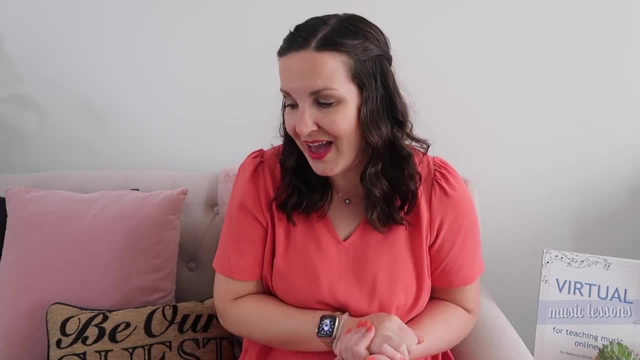 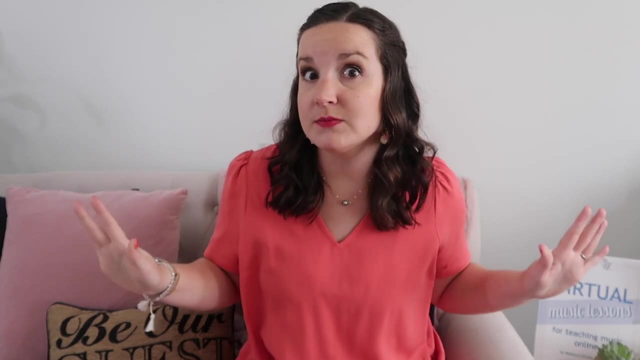 have a second way to do that. You can also add in different things. So, for example, you could have the kids pretend to move around like chickens on the A section and freeze on the B section. You have one kid chosen to move around on the B section. They're the only one who gets to move. 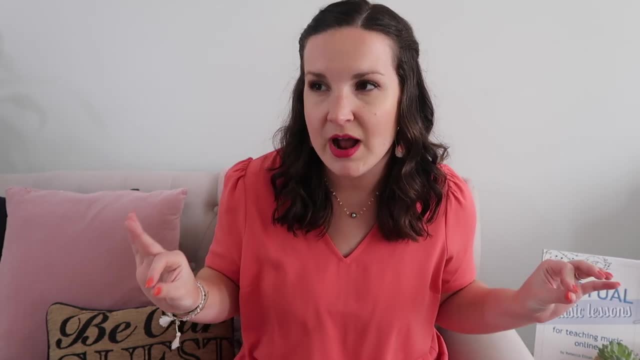 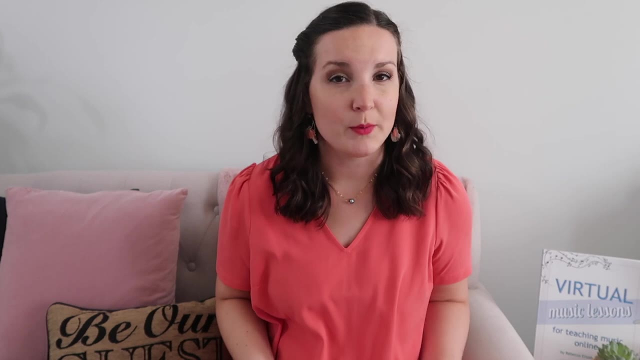 and everyone else is frozen. That's really fun And it can make this take a really long time because they all want to be in And so you have to keep doing it over and over and over. But lots of fun and really simple way to teach form again And that's a good way you can kind. 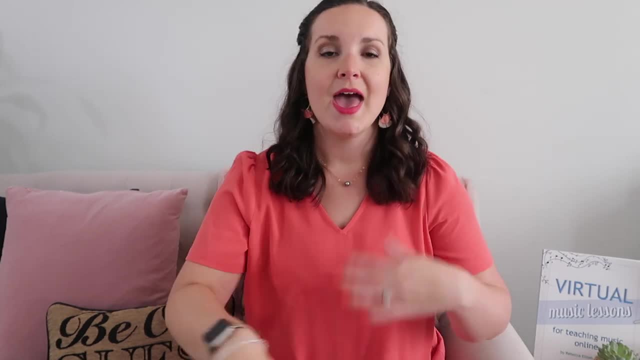 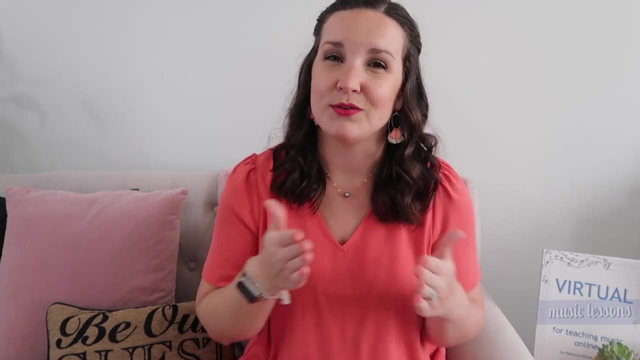 of start with. here's the letters, and then move to hands behind your back and then move to moving. You can even have them move in their seat, so they're not moving around, because you know six feet And also because I like to do everything stationary before we move around the classroom. 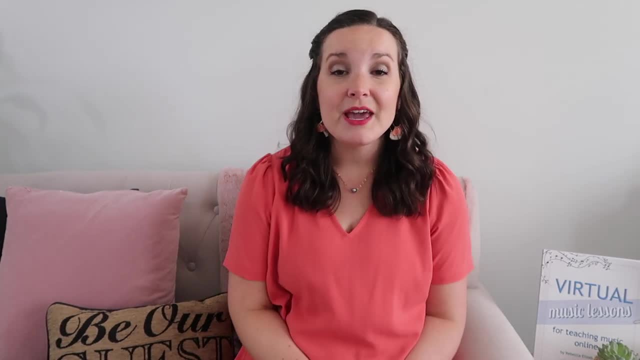 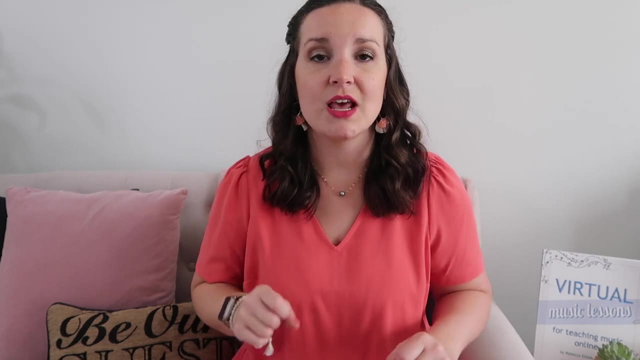 Because it just makes life a lot easier, And you can also add the parachute to this. So this is a really simple way to use the parachute. We just do like little waves on the A section and then on the B section. you can either have them walk around in a circle or you can just have them. 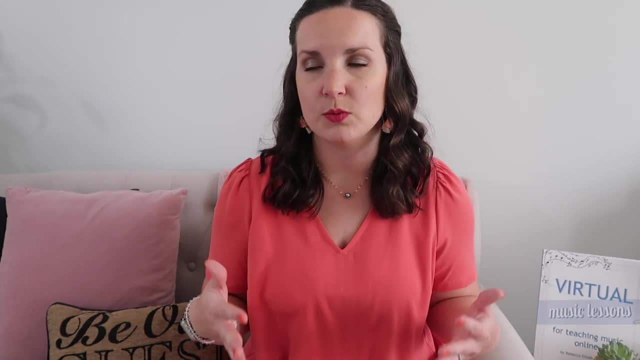 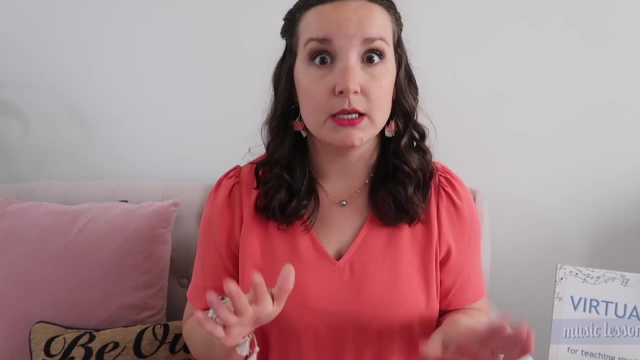 freeze And so really easy way again. to just see that form and it's super quick, super easy, Tastes like no prep. If you do not have a parachute, by the way, I'll link one down below. They are like game changers. They are amazing. You need one Number three. we're actually doing this one in. 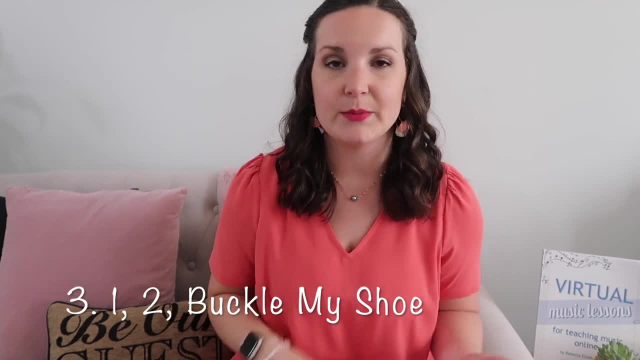 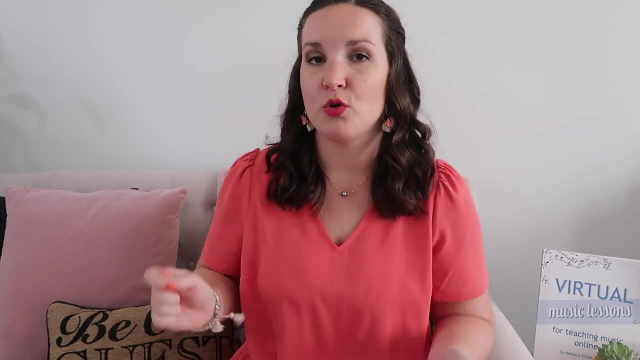 class right now and it is one to buckle my shoes. So this is a really easy way to do it. So if you really easy nursery rhyme again, I'll just kind of act out what we're doing. So we just do the numbers and then act it out. It's very simple. So it just goes: one, two, buckle my shoe. three, 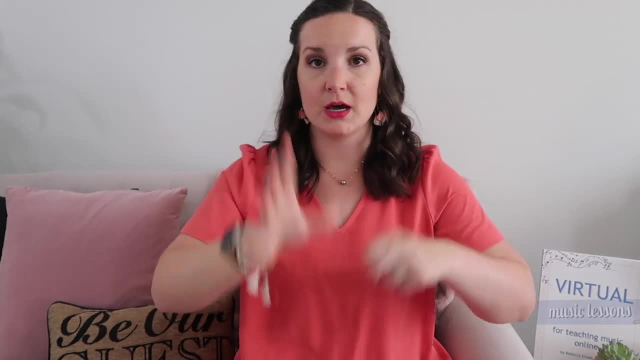 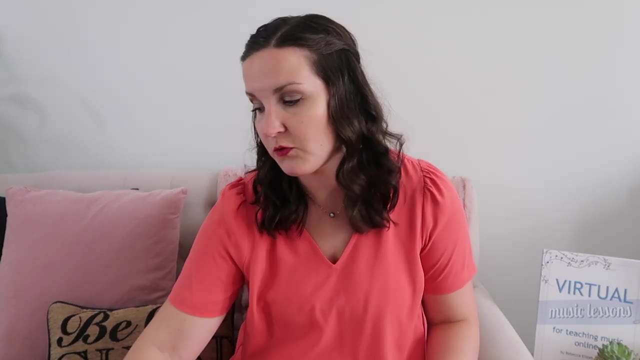 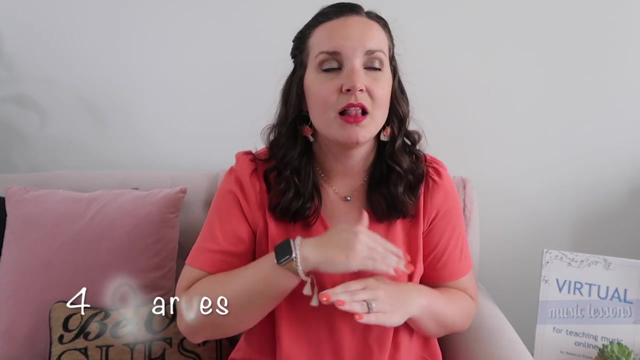 four, shut the door. five, six, pick up sticks. seven, eight, laid them straight. nine, 10, a big fat head. This would entertain them for quite a long time. And I also have a freebie that I will leave linked down below All right. next up is scarves. So I love using scarves in 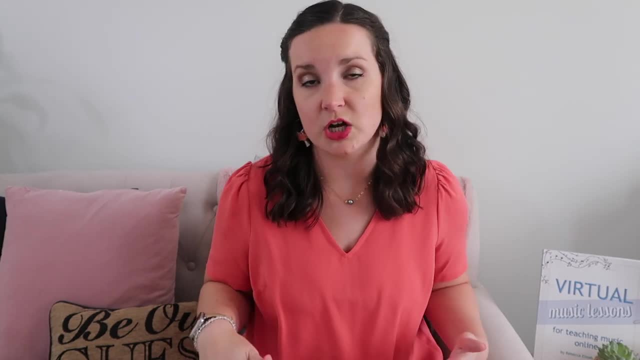 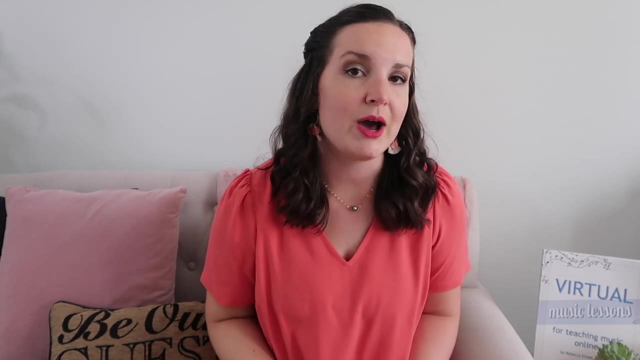 my elementary music classroom. We use them a lot. I love using them in my elementary music classroom All the time. The simplest way to use scarves, especially with little kids, is to have them either show the music or respond to contrast. So specifically we often do high and low and like. 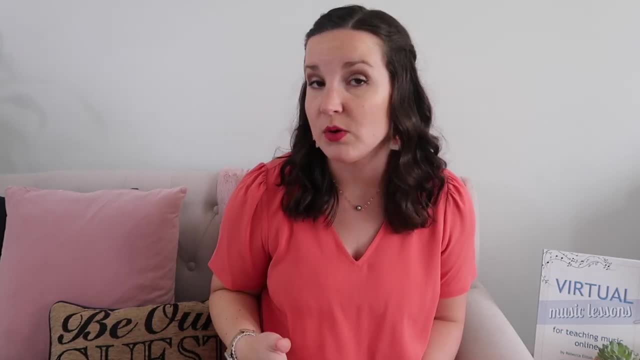 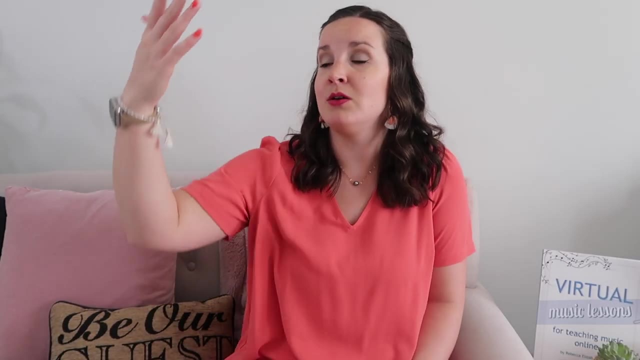 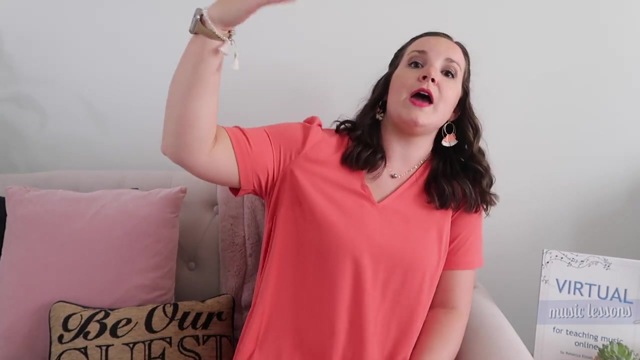 use the scarves to show the contour of a piece, A great one, for that is O Mio Babino Caro, because it's very dramatic And, if you're familiar, it has that like octave jump, So it's like down way up, and then it comes back down. It's super. 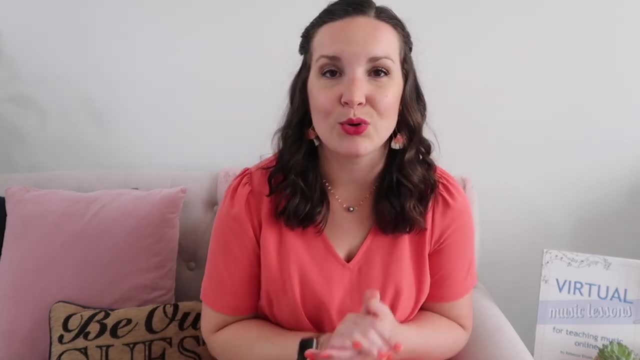 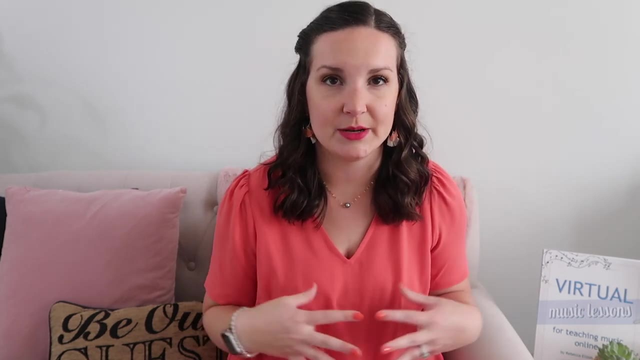 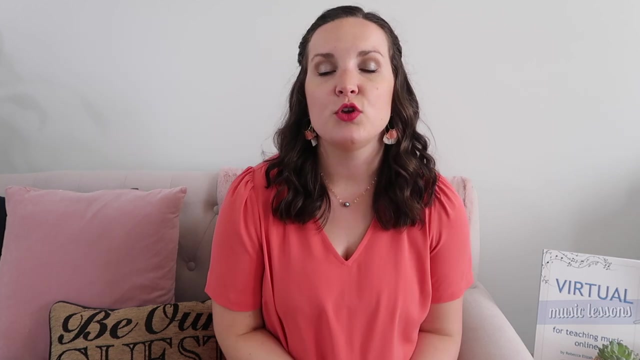 dramatic, super fun. The kids love it. So O Mio Babino Caro is a great one for that. I also like Bidlo is a good one for if you're doing forte and piano, And so I have the kids move small when it's piano and then big when it's forte If you want to have them just like. 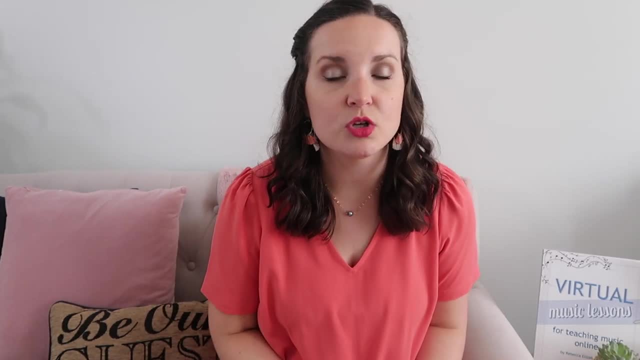 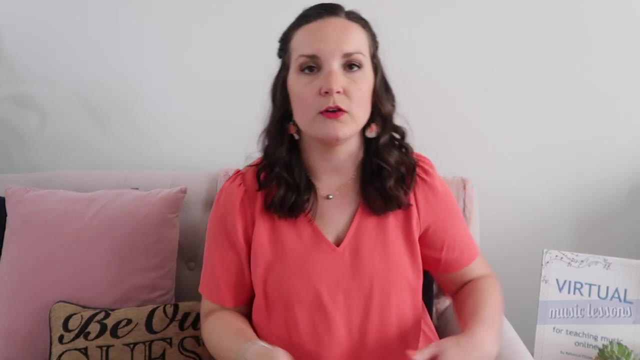 show the music. a good one would be Aquarium from Carnival of the Animals by Camille Saison, And so that one is very obvious, Like it feels like it's moving around in circles or it feels like it's going up and down. So it's a good one for that. And then I also have a good one for 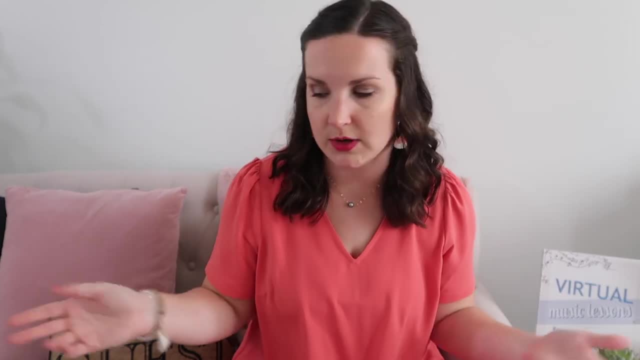 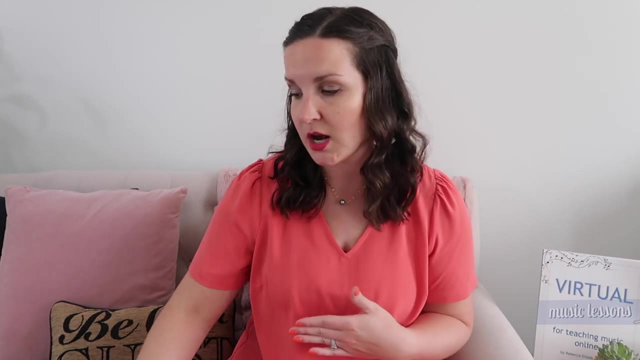 up and down, And so it's really easy for the kids to just show you what the music is doing. If you want something more structured, you could again go with form, and you can pick pretty much any song that has a distinct form and assign actions to it. One of my favorites is to do: 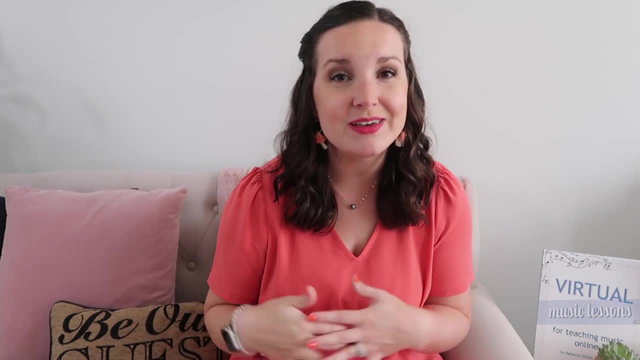 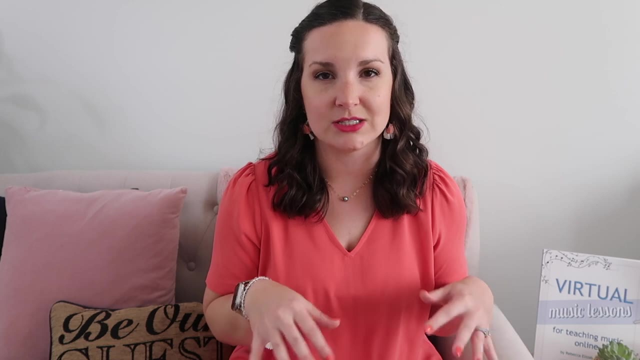 the song Le Toreador from Carmen. I love Carmen, I love this piece. It is so much fun. We have a whole thing for the upper grades that I will leave down below that you can see like how I use that. I have like four different ways that I use it with the older kids, But the younger kids 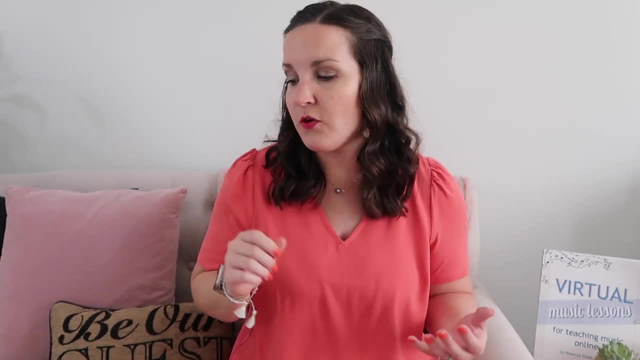 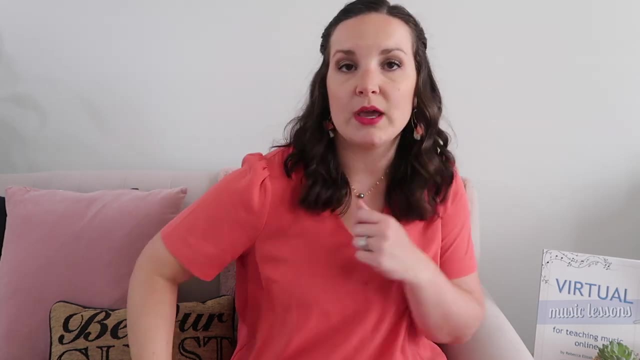 we will often do this scarf routine, And so for the pattern is A, A, B, A, C, A, And so for this, on the A section, we march with the scarf in our hands. When it comes back the second time, I tell them to move their scarf up and down like a baton. 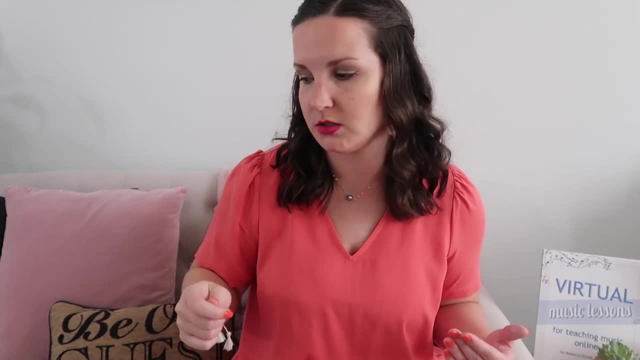 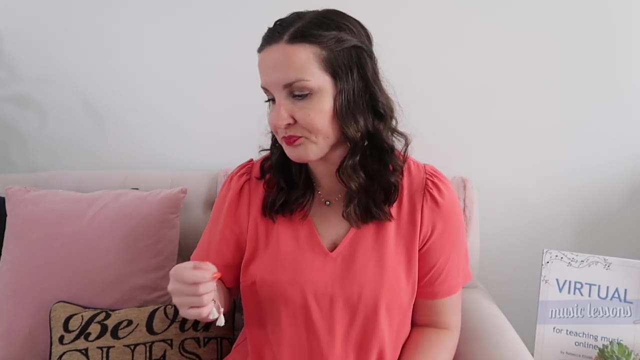 at the beginning of like a marching band- I don't know what that's called actually, because I didn't do marching band Anyway- and then on the B section we move the scarves back and forth above our heads for eight beats and then down for eight beats. We go one, two, three, four, five, six. 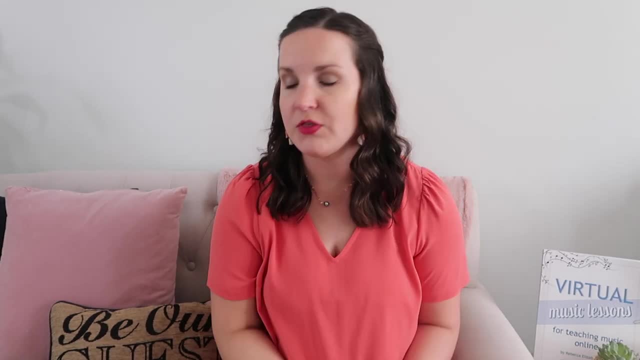 seven, eight, one, two, three, four, five, six, seven, eight. one, two, three, four, five, six, seven, eight, And we go back and forth And there's a lot of trills on. I think it's the. 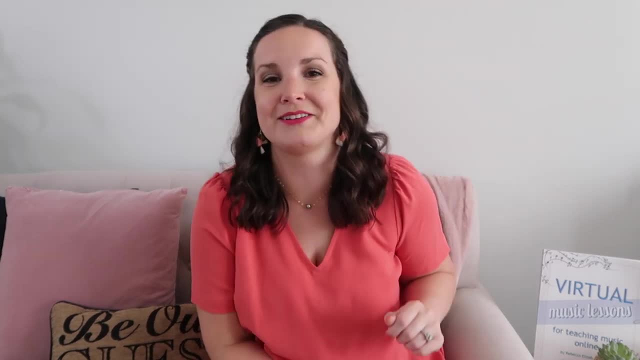 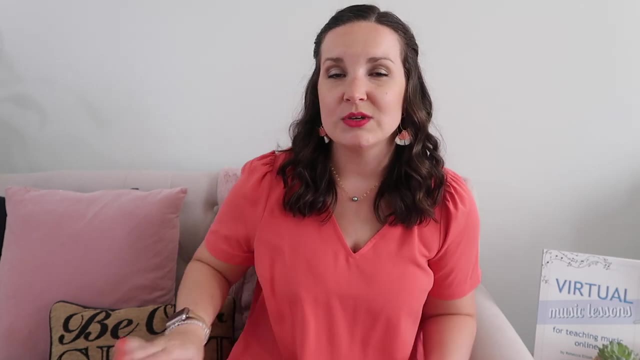 piccolo playing the trills And so for that you can just do like, so the kids can kind of get a feel for that. On this C section we're doing infinity signs. So I tell them a sideways eight and we start really, really low And you'll hear it does kind of like four different sections. So 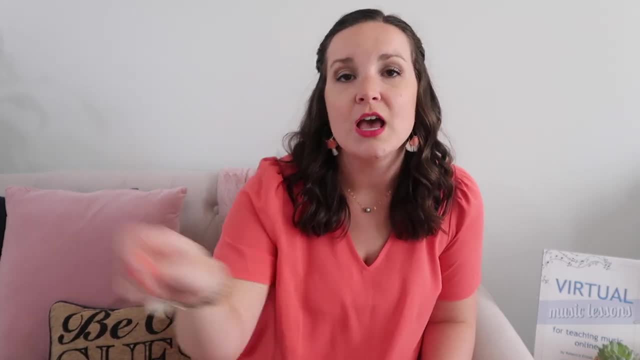 it gets a little bit louder and a little bit louder and a little bit louder. So we start all the way down at our feet with our figure eights And then, when it gets a little bit louder, we come up until we're all the way up at the top And then it goes straight back into 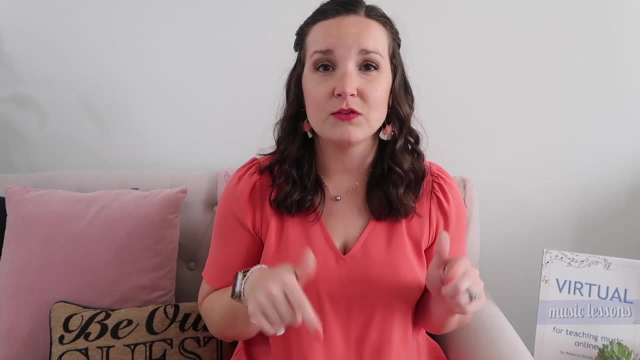 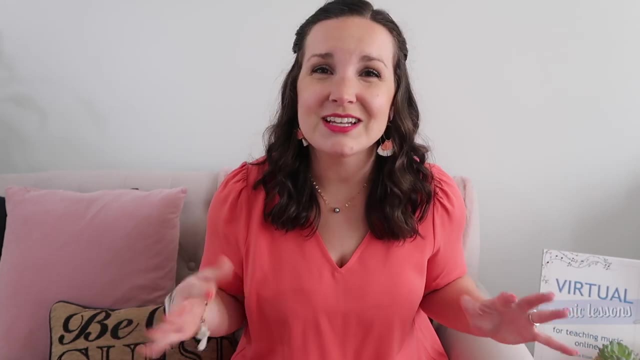 a March at the end with the A section. So highly recommend. I will leave a blog post down below that you can like see that again and see it like laid out in words. So it makes a little more sense. but that's kind of the gist of it. It is super fun, Highly recommend. highly recommend anything. 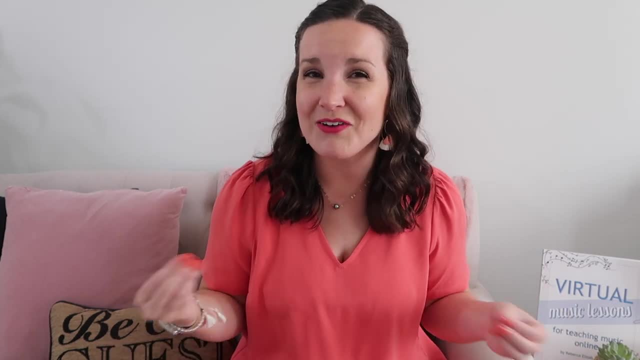 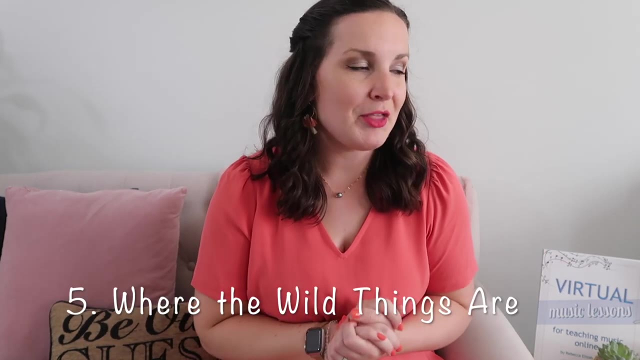 with scarves. I talk about scarves a lot, If you haven't gotten it, if you haven't figured that out yet. So definitely always a hit, All right. Next one is where the wild things are. So I bought the book where the wild things are a an embarrassingly long time ago, maybe two, three. 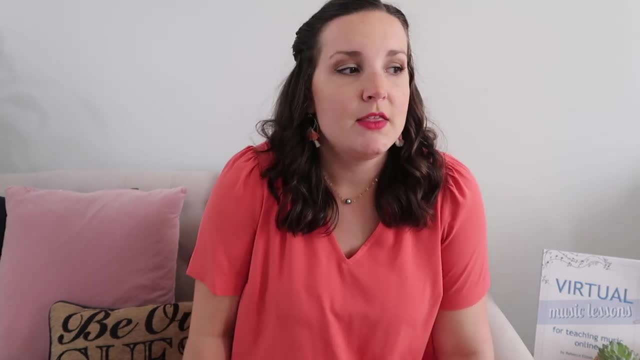 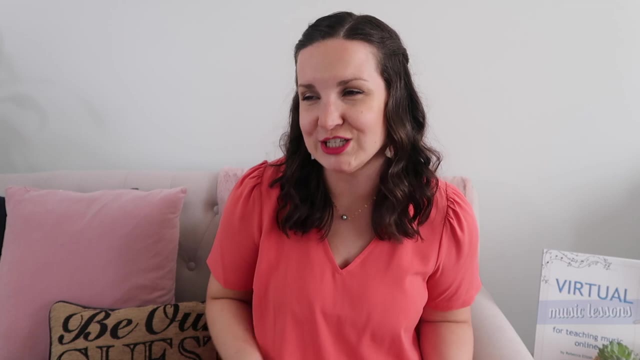 It's been a long time. So I was like, Oh, I would love to use this in music, And then I couldn't think of a way to use it in music class until now. So I finally sat down and actually thought about like what we could do And I came up with a whole set of lessons. So leave that link down below: We. 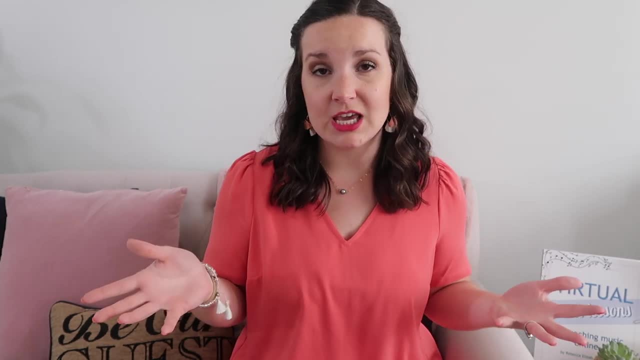 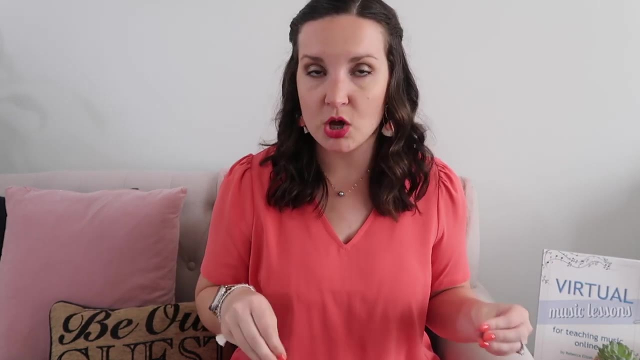 are going over rhythm in that one, So you can check that out. but specifically in there, along with all the rhythm activities, is a movement activity. So this is a free video on YouTube. I will link it below as well. There's going to be a lot of links. I will try to get them all. 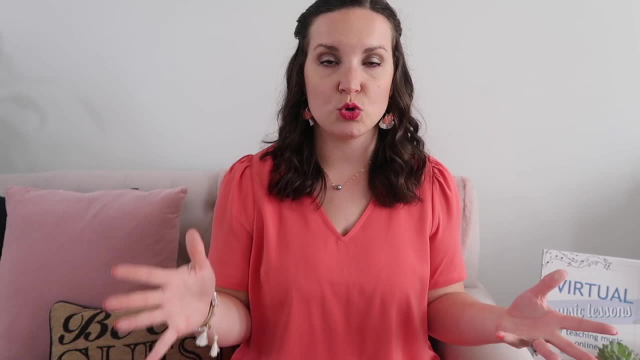 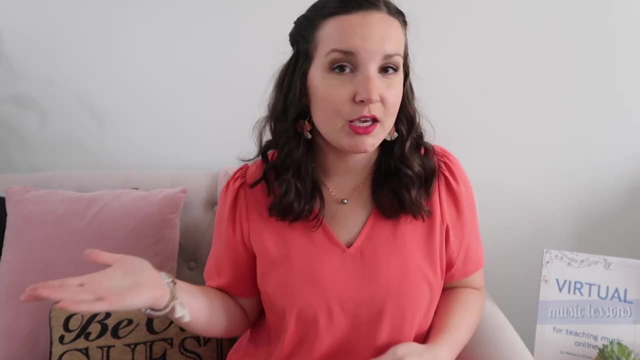 but basically the kids just watch the video And it tells them what to do, And so there's just all these different things that are inspired by where the wild things are. So some of the things include, like showing your claws or sailing away, like Max says at the end of the book, or just different things like that, so that you can kind 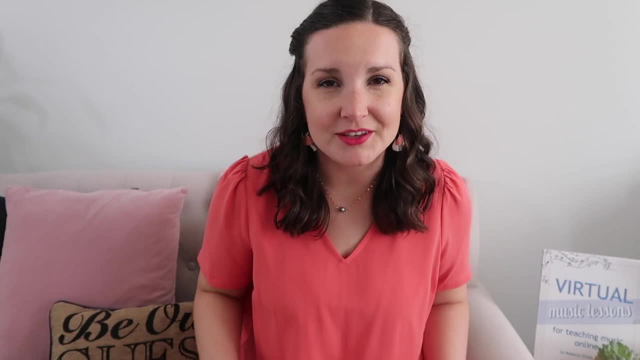 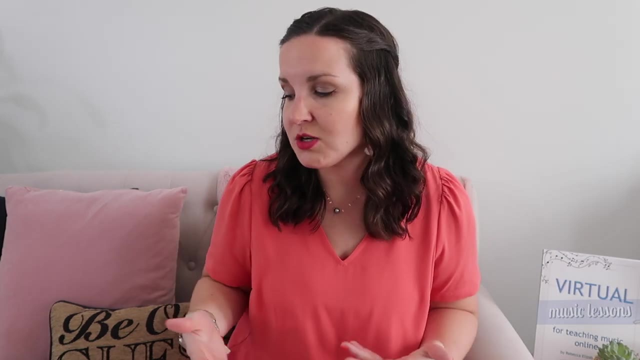 of like get that wild things idea, that wild things theme along with it, even though it's it's not like from the book, So very much inspired by the book but not actually from the book. And again, that's a really easy: you can just like pop it up on the board and the kids can do it. 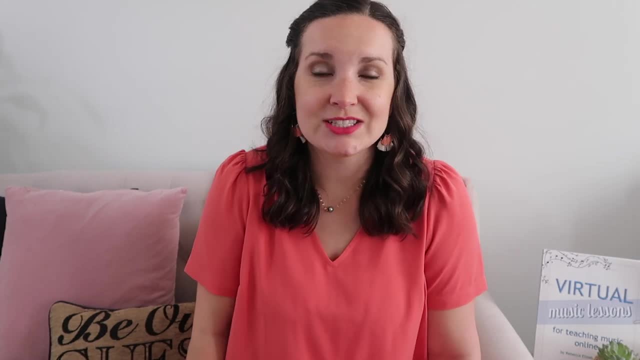 And it's super, super easy. It's lots of fun. All right, The next one is a song, and this is called walk and stop. I love this song. We use it a lot, And specifically we use it at the beginning of the year because 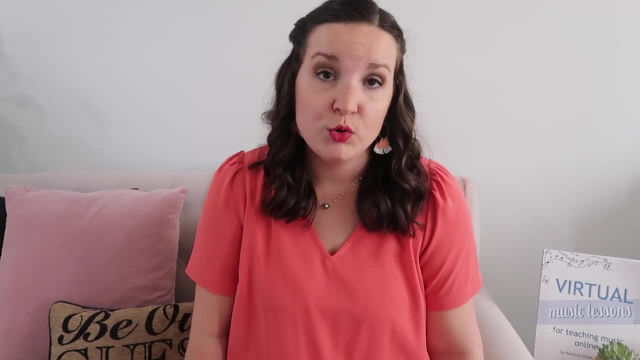 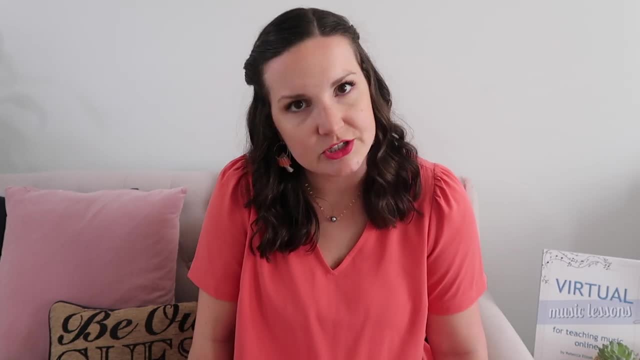 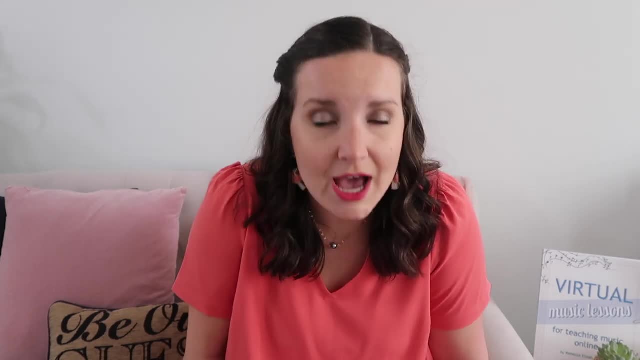 Or we might pat, or we might stomp, or we might jump or we might hop, whatever gets the wiggles out. This is one of my favorite go-tos, and you can have the kids pick what actions we're going to add to it. 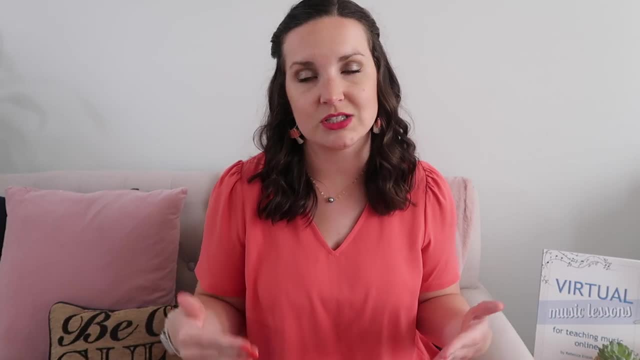 And it's just tons of fun. You can have it locomotive, move it around the classroom or you can have them just stay in their seats. Either way, tons of fun, highly recommend. The next one is we're going on a bear hunt. 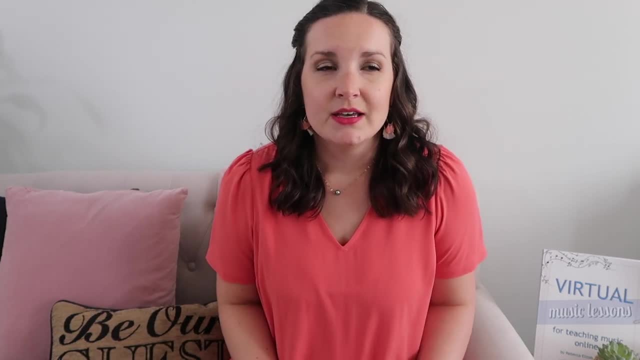 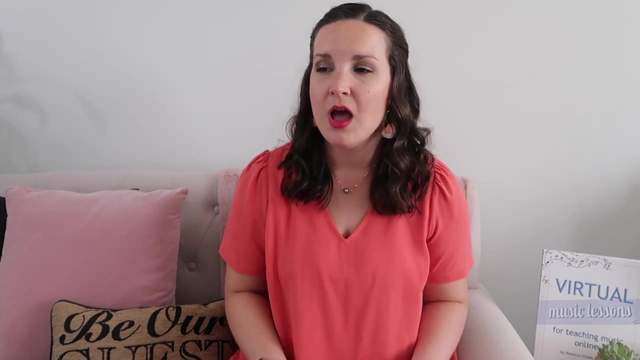 So if you are not familiar with this one, it is a. it's a song and it's also a book, I believe. I did some research and I think the song came first, but it's hard to tell, honestly. Basically, you're going hunting bears and you come up to all these different obstacles. 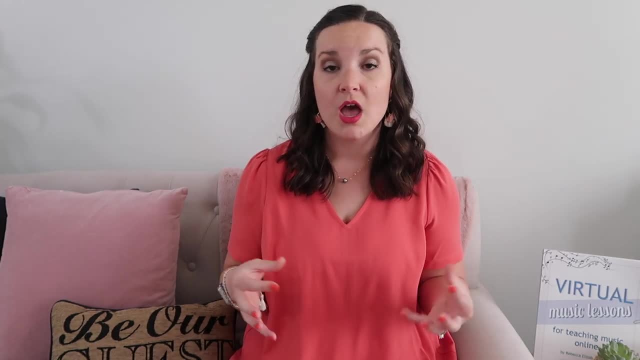 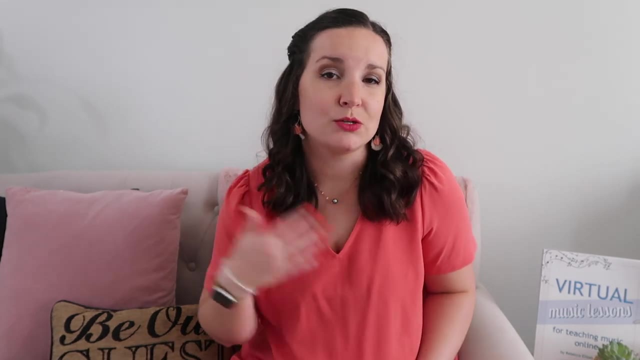 So I'll leave a link to the video of the guy who wrote the book doing like I'm doing it all out for you if you don't want to lead it. but also you can do it yourself. And so what we do is we keep the study beat and it's a repeat after me song, so they just echo back to you. 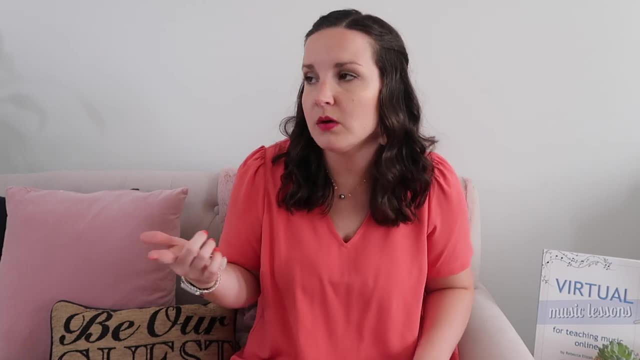 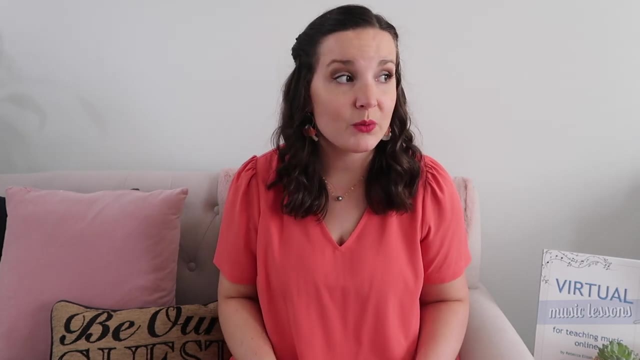 So we do. we're going on a bear hunt. we're going on a bear hunt. we're going to catch a big one. What a beautiful day. I'm not scared, I'm not scared. And then you come up to all these different things. 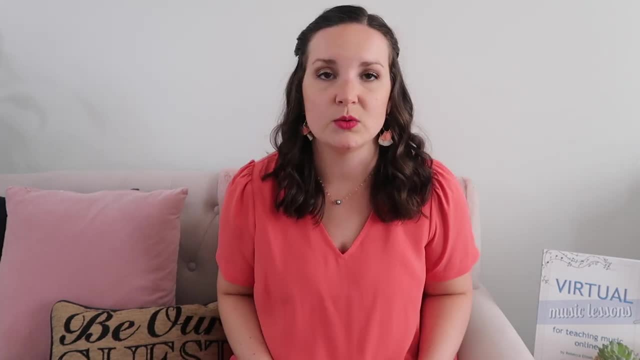 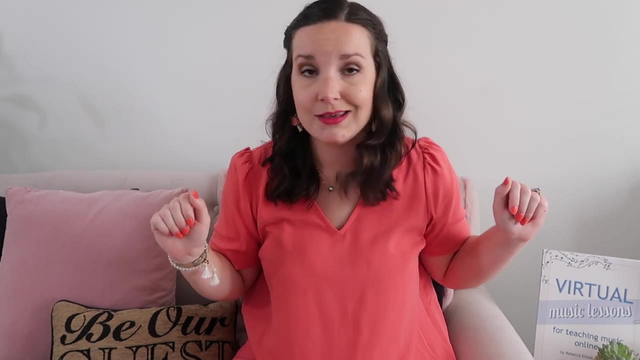 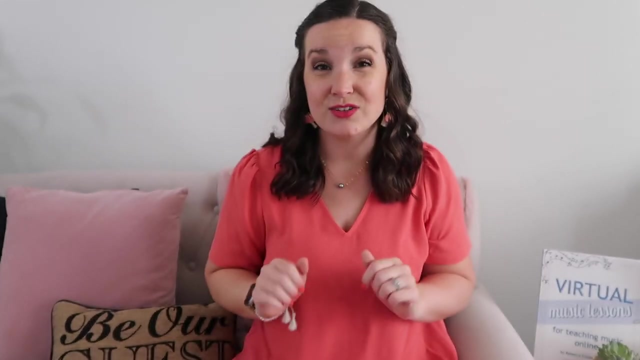 So we always do the tree. So, like one of them is the tree, So we might do. we're coming to a tree, a big, tall tree. can't go under it, can't go around it, can't go around it. I have to go over it. I have to go over it. woo, woo. 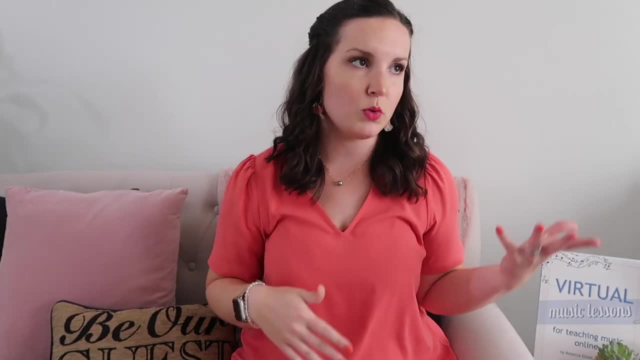 woo, woo, woo And we go through all these different things. So we go through like the mushroom patch, We go through the river and we go, We go over the bridge, We go through all these different things And it's also a really good warm up because it gets their voices like doing all sorts. 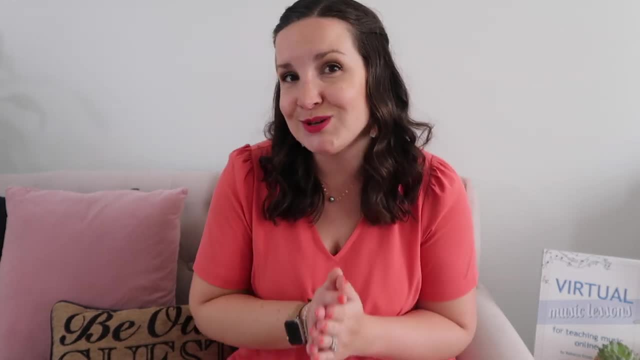 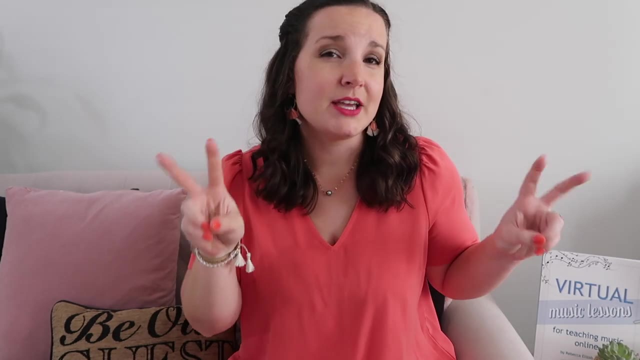 of funky things. It's super cute, Super fun. The kids always love it And you can make it even more fun by going around the room- So I've done this before- where I'll set up different areas So I might put, like, some blue fabric down to be the river that we swim through. 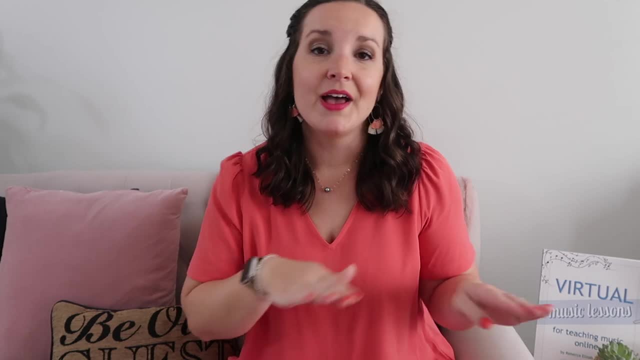 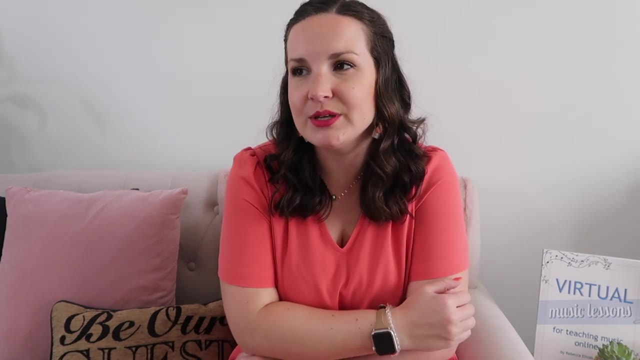 Or you might put like little like rocks on the paper down that they have to go through, Or I'll make like a tunnel that they have to go through, Or like a tunnel that they have like underneath the tables and just all these different things, and have them kind of go like in a line and going through all these different things. 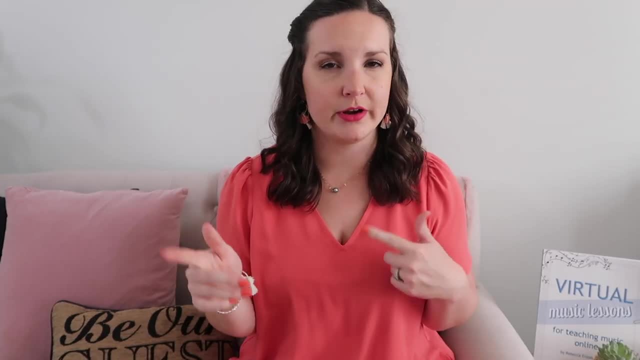 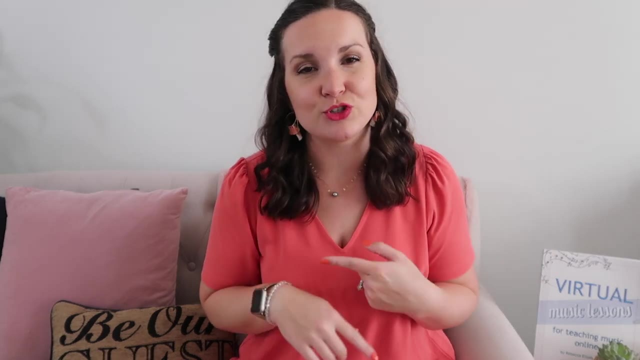 And it is so much fun. This is included with Hickory, Dickory dock and a bunch of other things like grizzly bear, mouse, mousy and different mouse and bear things in my virtual field trip to the forest, So I will leave that link down below. 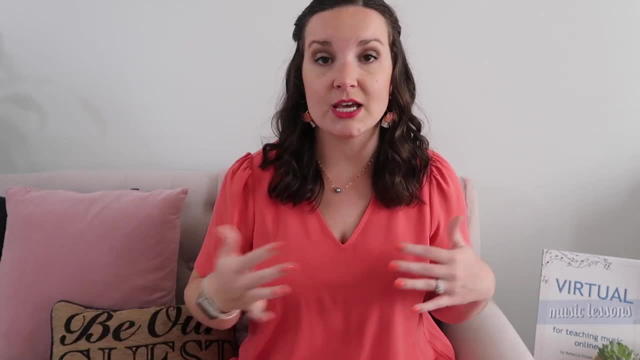 It's all about piano and forte, And so we're using the bears and the mice to teach piano and forte, and it has lots of different songs and stuff, So definitely check that out down below. All right, Let's talk about London Bridge. 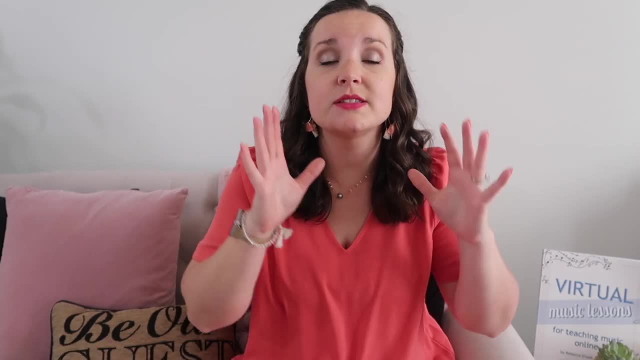 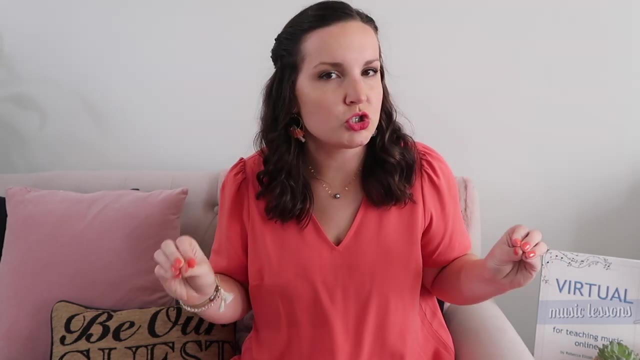 Now I know you're probably like Becca, seriously you're adding London Bridge on here, But London Bridge is such a good one that kids these days don't know Seriously. I know because I teach children's church in addition to teaching music and in children's 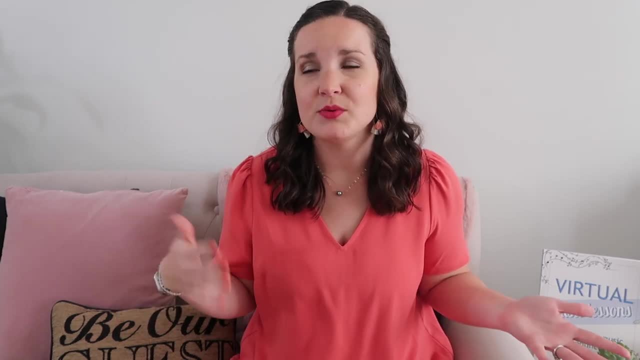 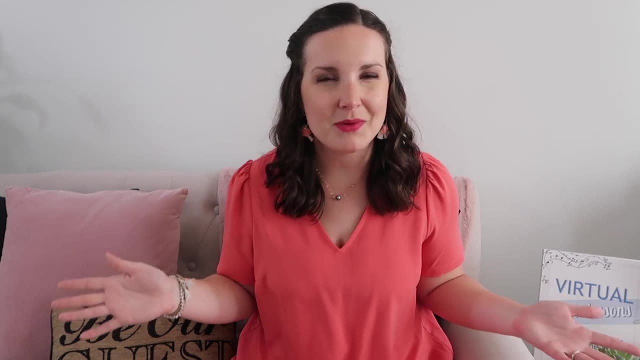 church the other day we were doing some lesson. I don't even remember what we were talking about, But it was something where I was like, oh my gosh, we could play like a variation of London Bridge, and then that would work perfectly, because they were going under. 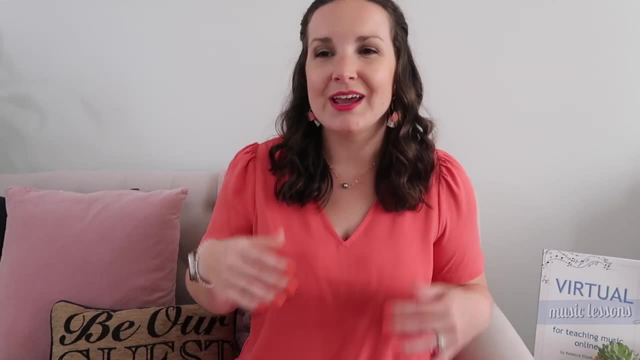 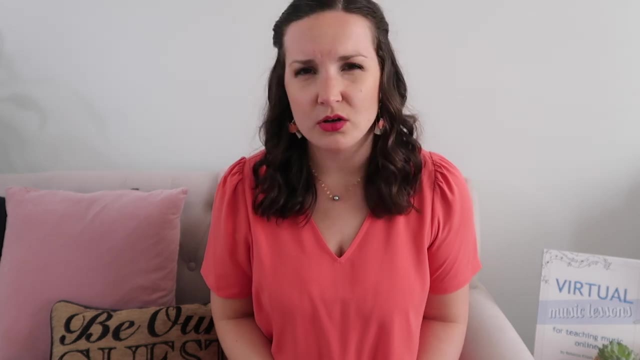 Maybe it was the Red Sea, part of the Red Sea, I don't know Anyway. and so we were going to do London Bridge And I was like who's playing London Bridge? And they were all like, and I mean like first or fifth graders, I was like you've. 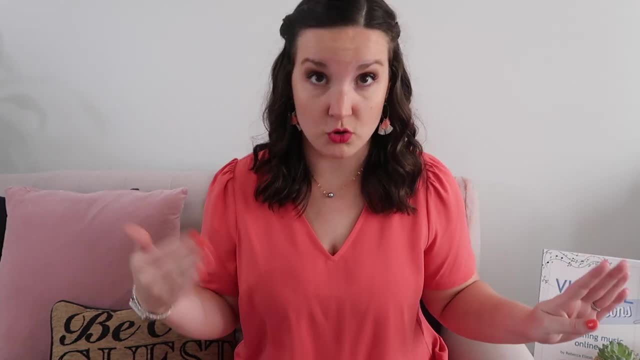 never played London Bridge before, So we played. so I was like: all right, well, first of all we got to play the normal London Bridge, So we played the normal London Bridge And they were like: this is so much fun, even like the 10 year olds. 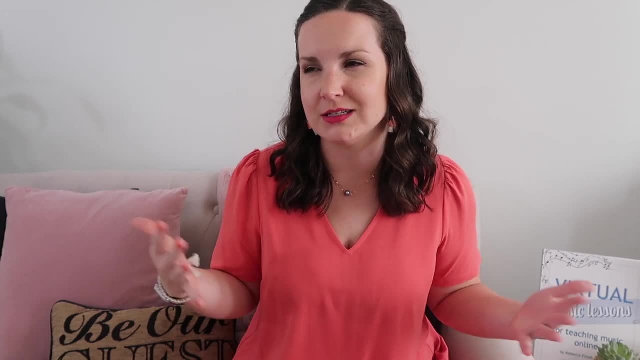 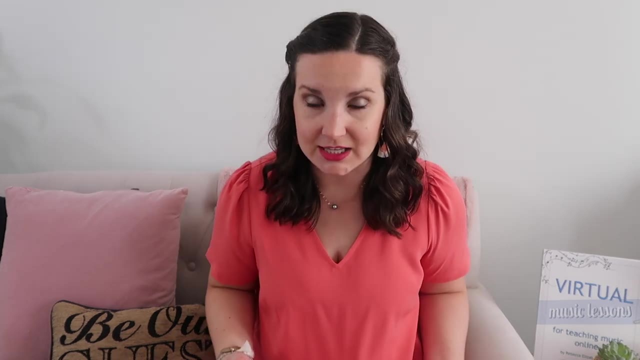 And I was like Yes, it is. And then we also played it And, however, I connected it to the Bible story, which I now don't remember anymore, But the point being it is so much fun And it's highly underrated. 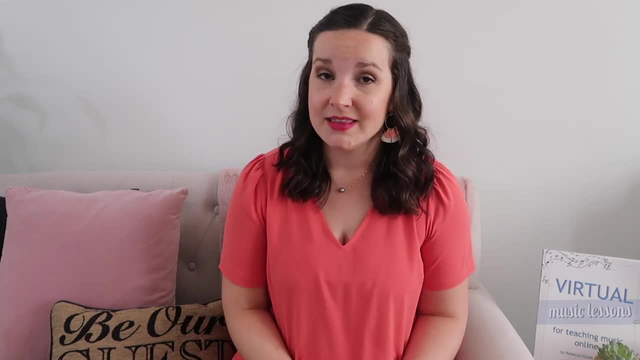 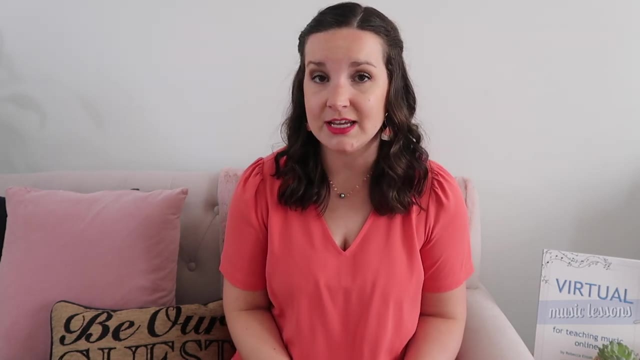 So if you don't know the story, And then we play the song London Bridge, It goes: London Bridge is falling down, falling down, falling down. London Bridge is falling down, my fair lady. And there's tons of different verses, But the other one that we do. so we do that one. 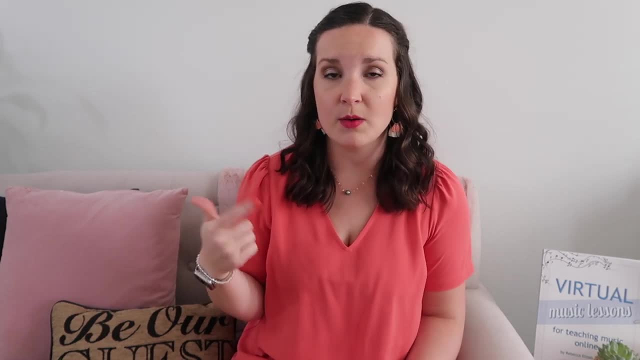 And we do a second one, which is shake them up with pepper and salt. So this, shake them up with pepper and salt, pepper and salt, pepper and salt shake up with pepper and salt, my fair lady. And so what we do is the kids walk around in a circle. 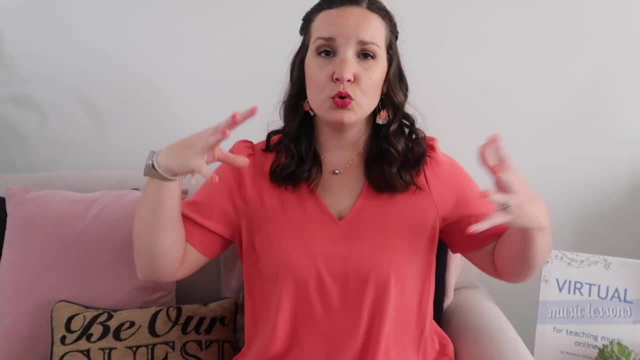 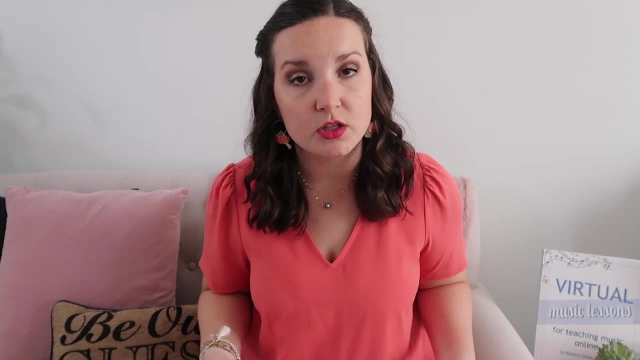 I usually have them walk on the edge of the carpet so that it's easy to get there. You and another student hold hands to make them walk, hands to make the bridge. whenever the song stops, whoever's standing under the bridge gets caught under the bridge, and then we do shake them up with pepper and salt, and so we'll, like you know. 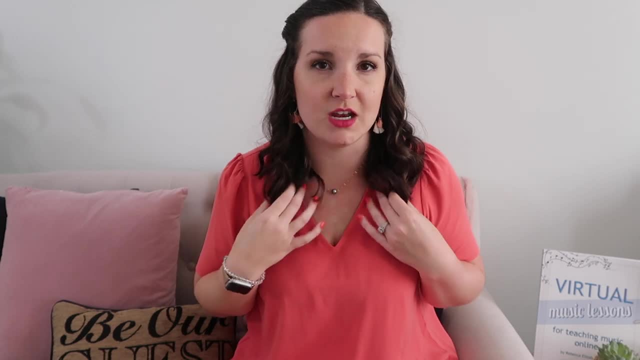 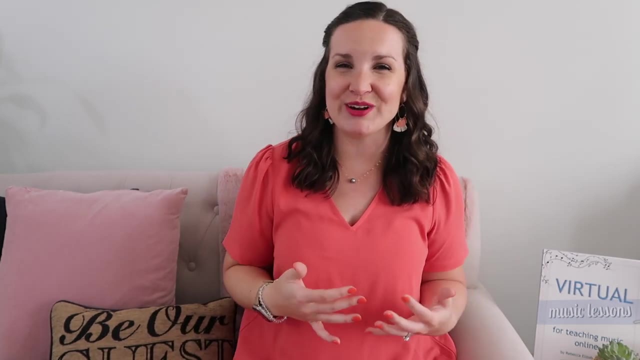 shake our arms back and forth, and that's why i always want to be in the bridge to make sure that the kid is, you know, safe, because i can make sure that we give them plenty of room when they get caught underneath the bridge and stuff like that. so i just always do myself and then another kid. 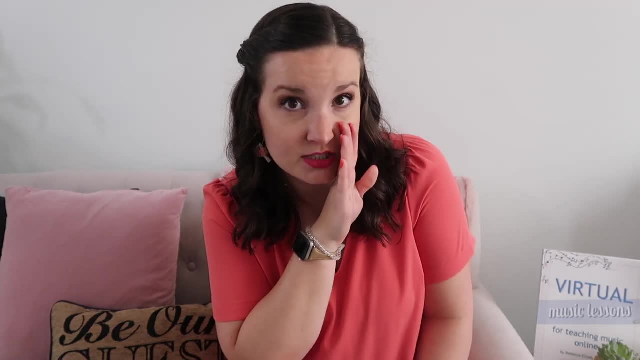 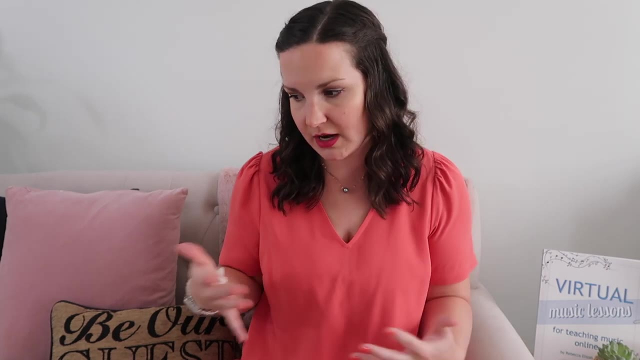 and usually if you have a kid that often causes trouble in class, that's a great one to pick because you can keep an eye on them and they feel special. so that also helps to kind of fill that up super fun. my kids love, love, love london bridge and it's super simple. you can play it if you're. 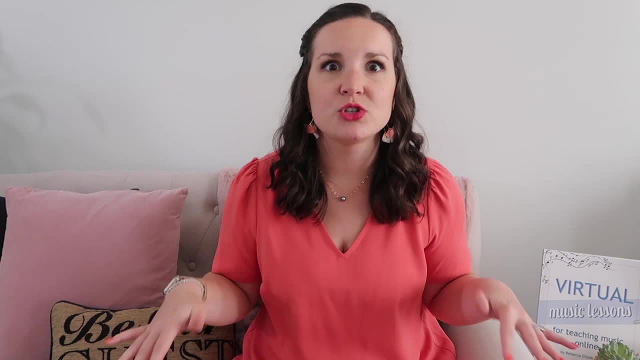 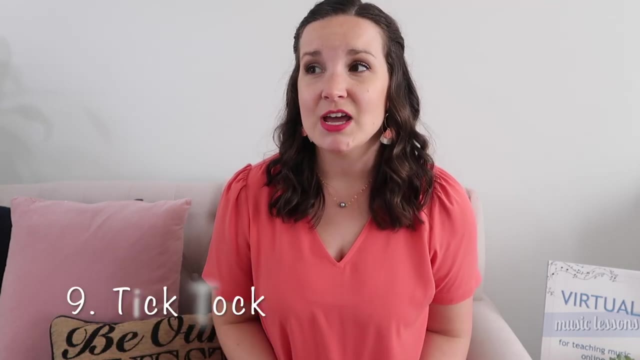 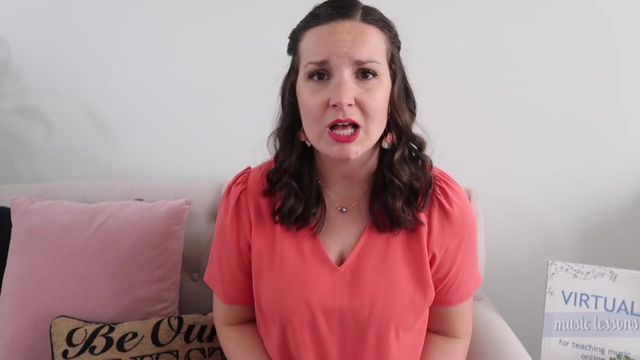 in their classroom. you play if you just got like an extra five minutes of time. so much fun, so much fun. they love it, it's so great. now a not so common song is the next one, and that is tiktok. i found this on youtube or on the internet somewhere, and it was like i had never seen it anywhere else, and 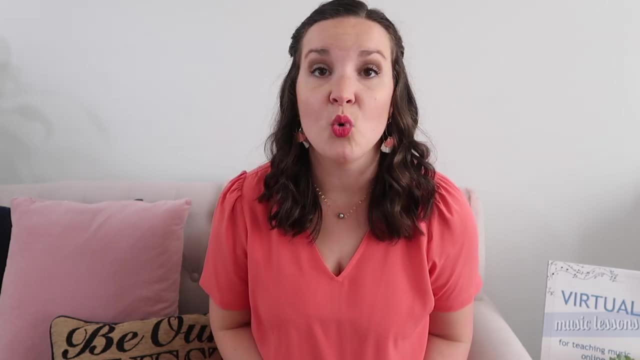 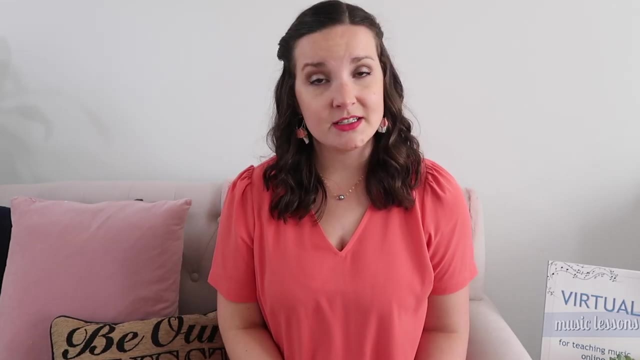 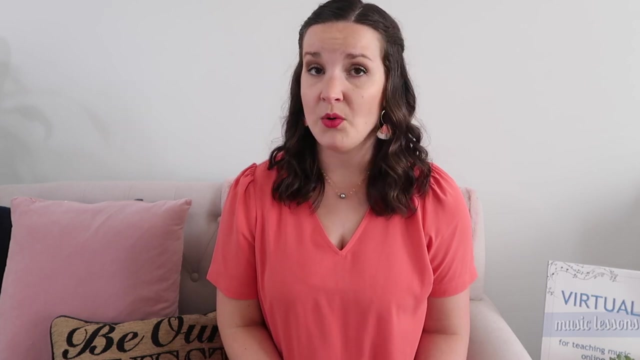 i can't even find the place that i originally found it. so all of that to say, it is still so much fun, but it's not super common. so this one goes tiktok, tiktok goes a little clock, night and day, it just goes tiktok open wide the. 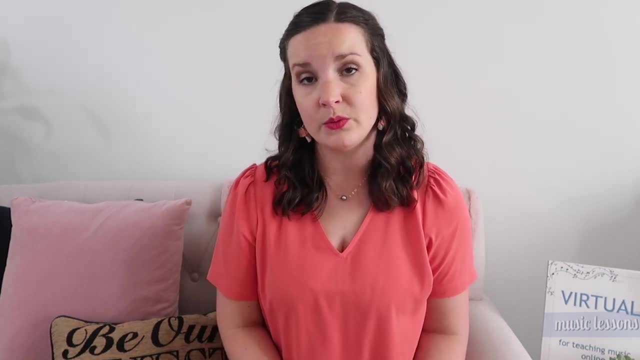 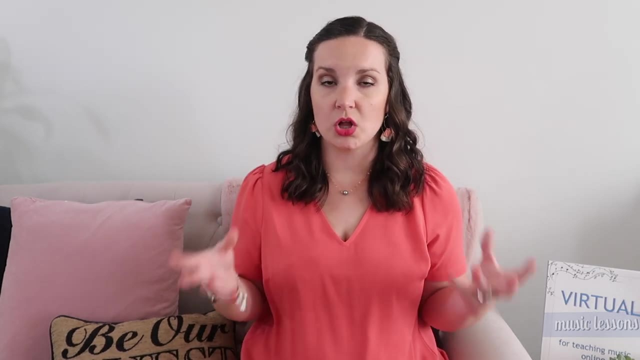 doors of the little clock. so we do this in partners, and so one person is the clock and then the other person does the clock, and then the other person does the clock, and then the other person does all the action. so they stand still. the other person walks around in a circle around. 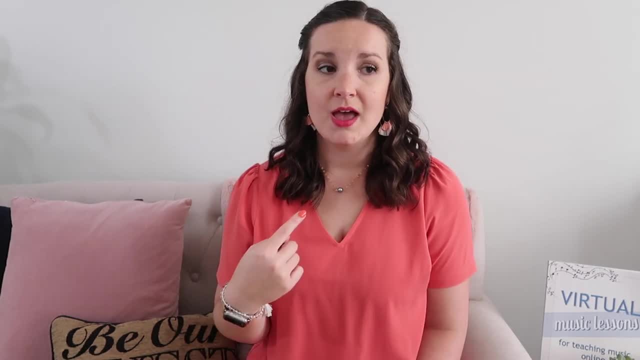 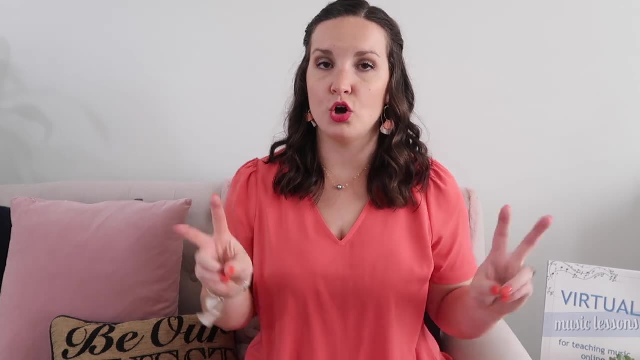 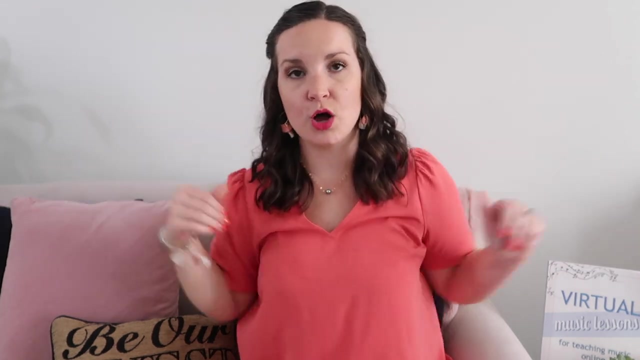 them. so they do tiktok, tiktok goes a little clock, night and day. it just goes tiktok. and then when it says open wide, they stand behind the clock and they open wide by pulling the kid's arm, not hard but you know, just pulling them up like this. and then the kid behind pops out when you say cuckoo. 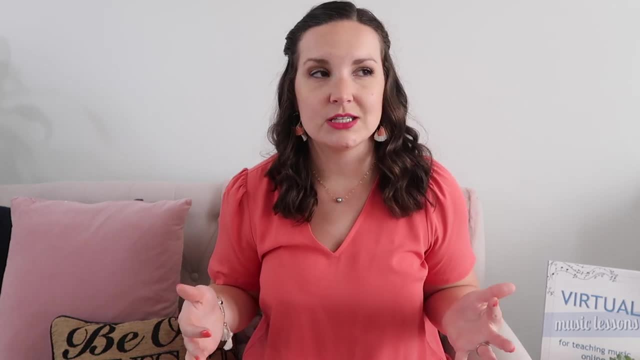 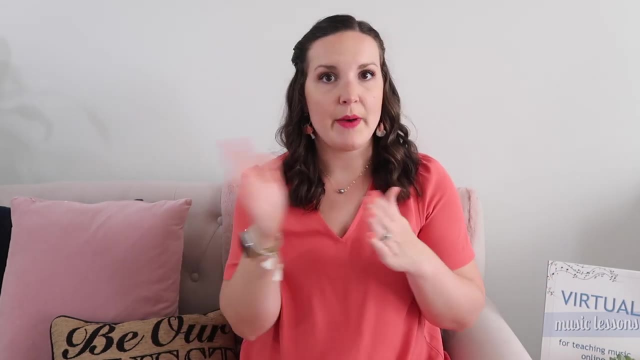 like, just like if you've ever seen the sound of music like that um at the end, when they're singing the so long for a while song and they do that um, so they just pop out from each side. so this is super, super fun. it does get a little bit difficult to get those, so i'd like to start it in place. 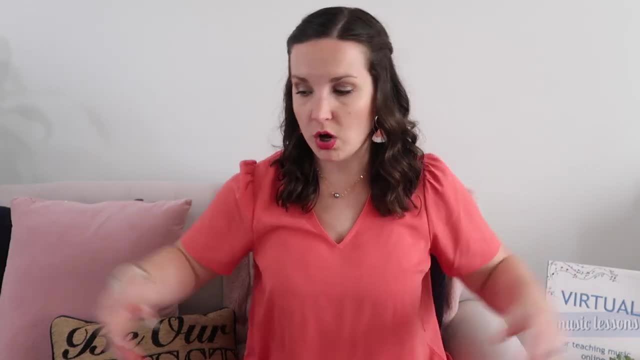 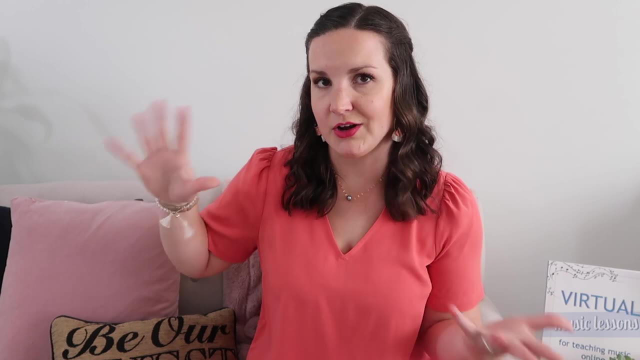 first. so for that i just have the kids walk. they open their own arms and then they go to the sides for cuckoo. so it's pretty much the same thing, but without the partner. and then we have the partner and they already kind of know, and they know the song and all that good stuff. so little hack for.